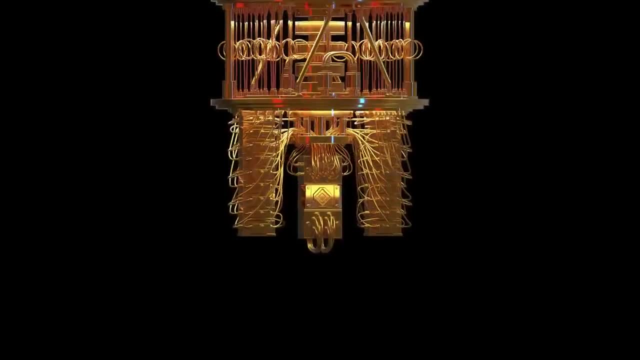 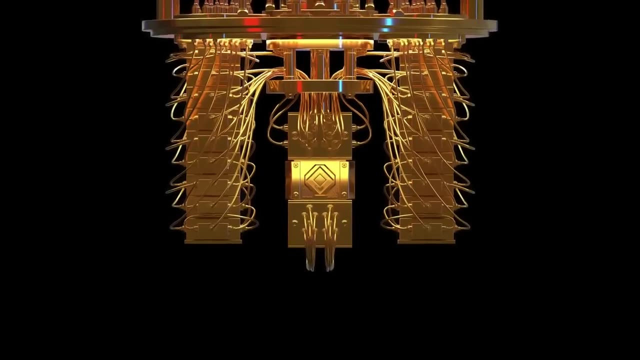 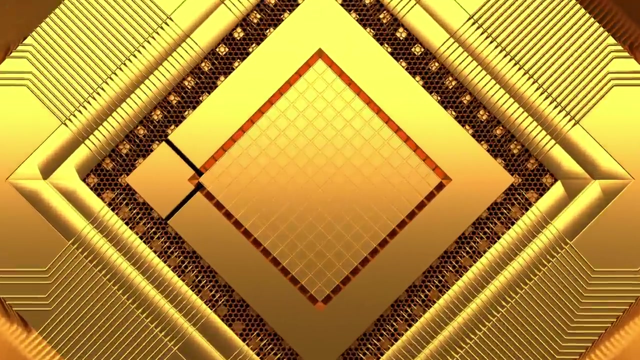 aren't the next generation of supercomputers. They're something else entirely, And before we can even begin to talk about their potential applications, we need to understand the fundamental physics that drives the theory of quantum computing. We'll need to dive into another dimension, smaller and more alien than anything we intuitively understand. 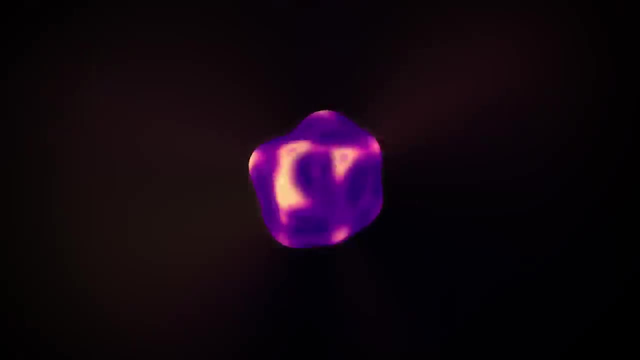 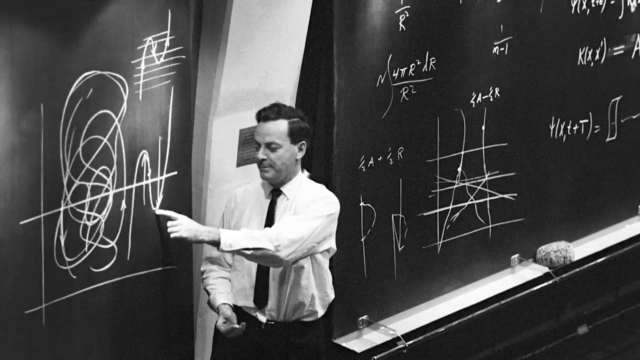 the subatomic world of quantum mechanics. In the 1980s, one of the most important physicists of the 20th century encountered the problem of quantum mechanics. In the 1980s, one of the most important physicists of the 20th century encountered 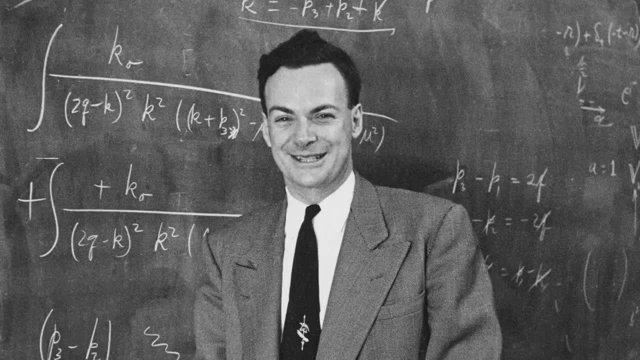 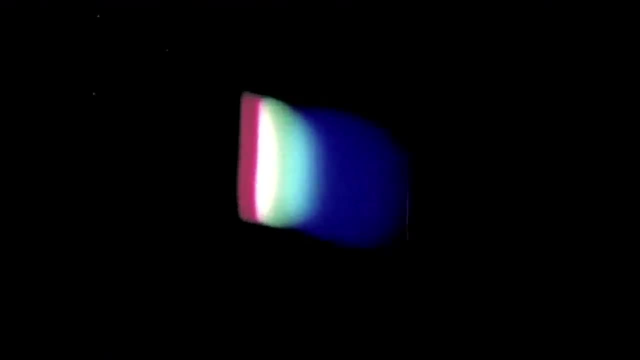 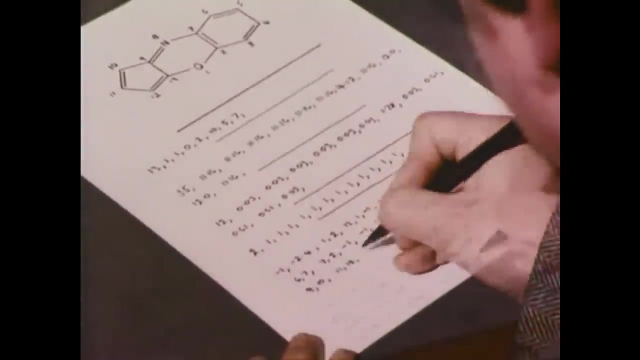 a major roadblock. Richard Feynman was hungry for a window into the quantum universe, But quantum systems by nature are fragile and the information they hold hides from us. Because Feynman couldn't directly observe quantum events, he wanted to design a simulation. It quickly became clear that his computer 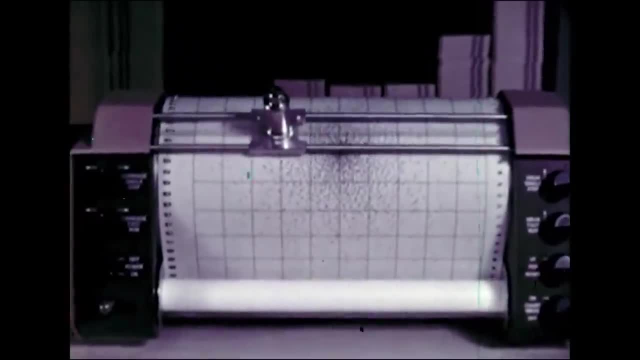 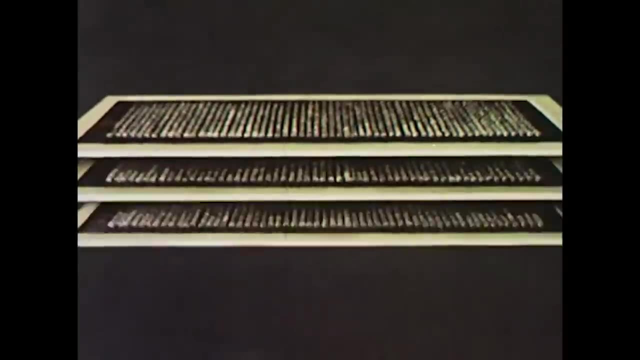 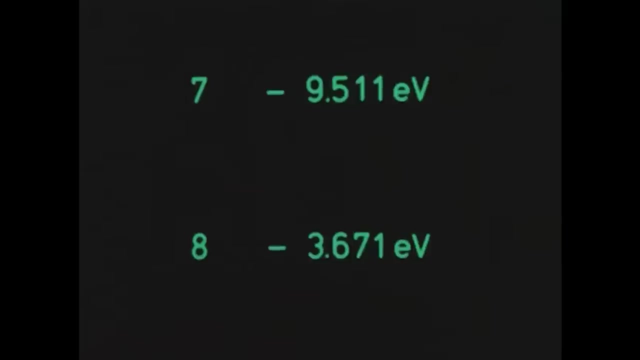 wasn't up to the task. As he added particles to the quantum systems he was modeling, the cost of computation began to rise exponentially. Feynman concluded that classical computers just can't scale up fast enough to keep pace with the growing complexity of quantum calculations. Then he had a breakthrough. 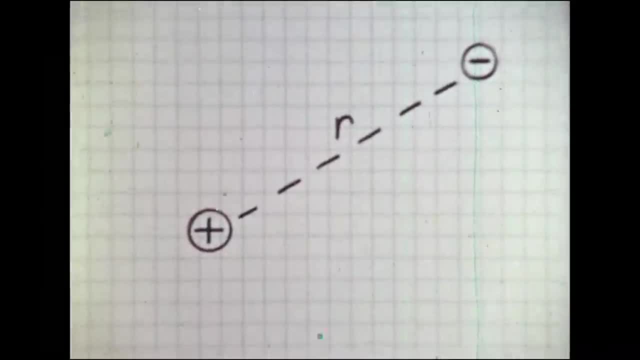 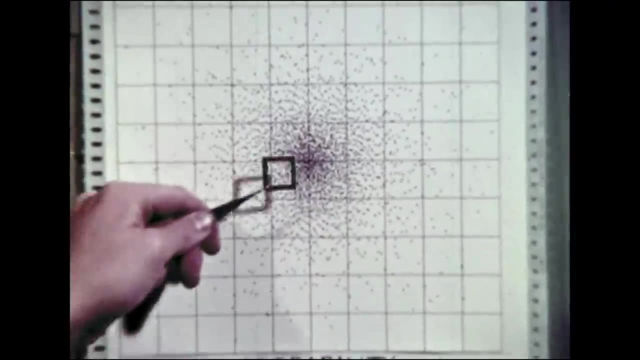 What if he could design a tool made up of quantum elements itself? This instrument would operate according to the laws of quantum physics, making it the perfect way to probe the mysteries of the quantum realm. The idea of the quantum computer was to create a system that would be able to predict the 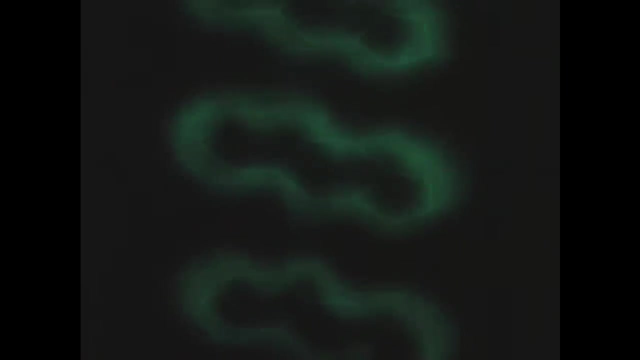 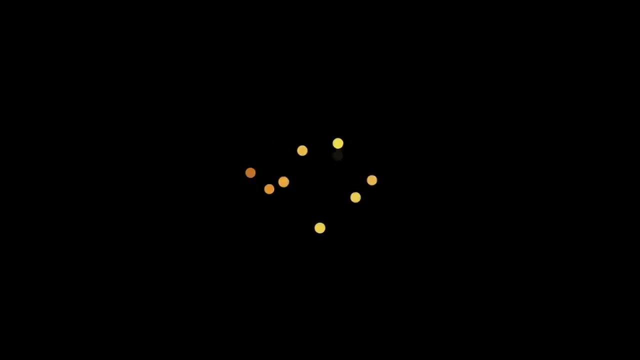 future of quantum physics. The idea of the quantum computer was born, And by dreaming it up, Feynman had started to build a bridge between quantum physics and computer science. To understand how quantum computing works, it's essential to start by understanding what makes it quantum in the first place. This means 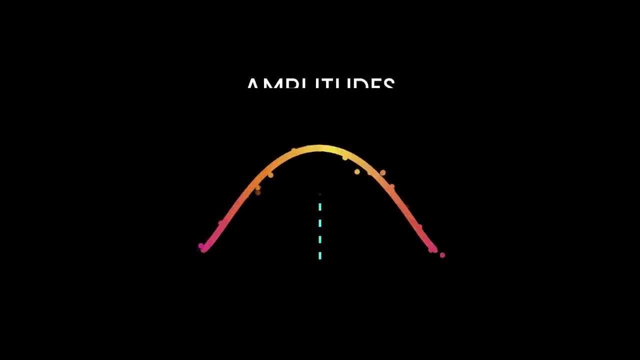 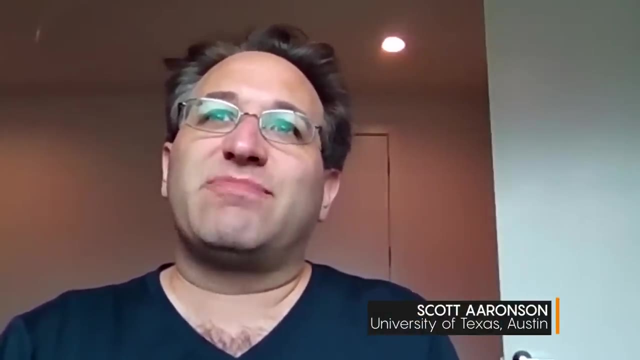 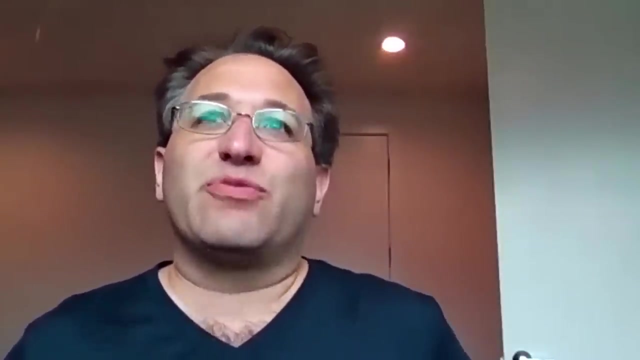 that we need to talk about what's at the heart of quantum physics, a concept called amplitudes, Quantum mechanics. at its core is a change to the rules of probability, And this is also where the power of quantum computing comes from: from these different rules of probability than the ones that we are used to. 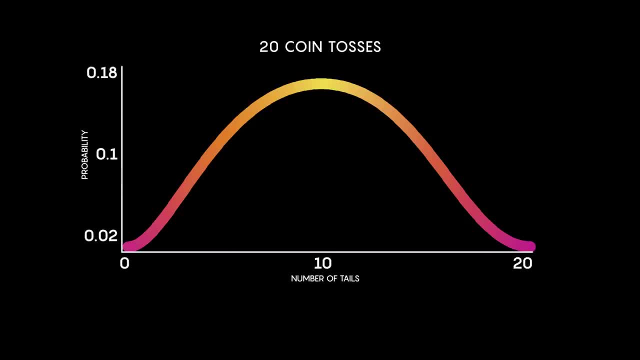 For example, if you want to know the classical probability of an event- say a coin landing tails exactly 10 times out of 20, you add up the probabilities of all the different ways that event could happen. That's just common sense. But common sense doesn't govern the quantum. 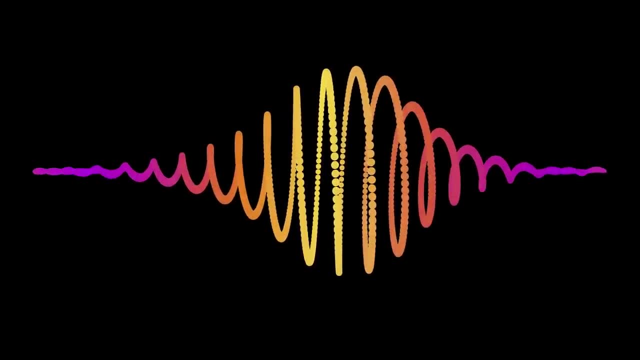 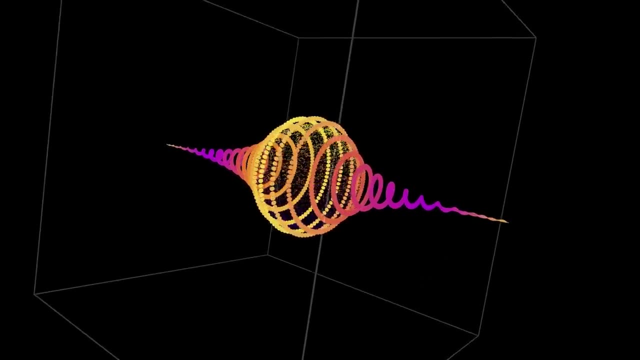 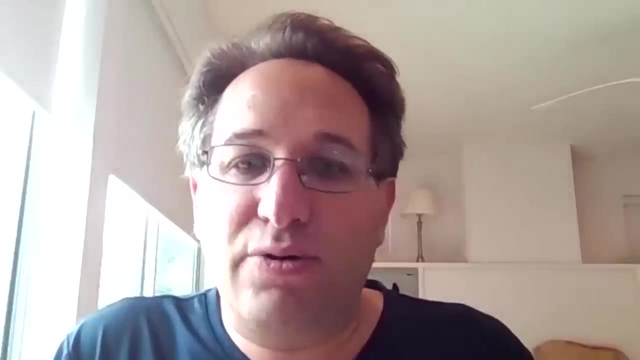 universe. Before you measure a subatomic particle, you can think about it as a wave of probability that exists in a kind of black box, a quantum system with many different chances of being in many different places. Amplitudes are closely related to probabilities, but they're not. 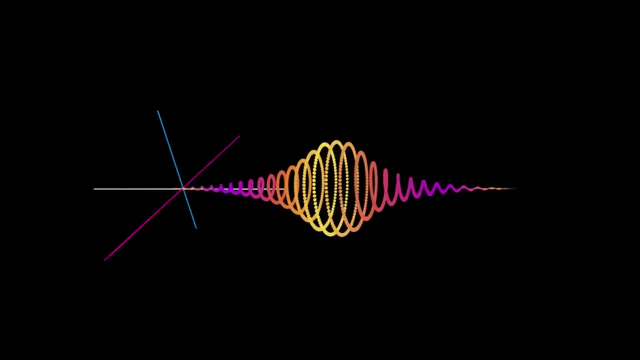 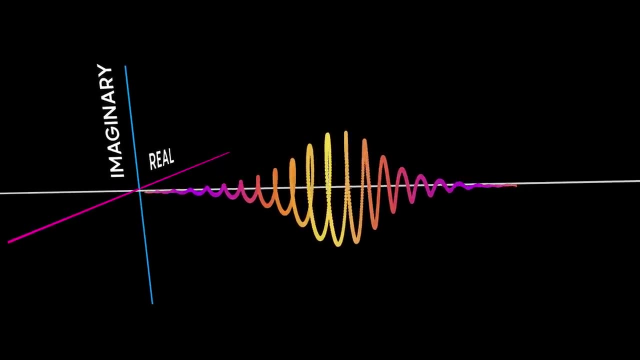 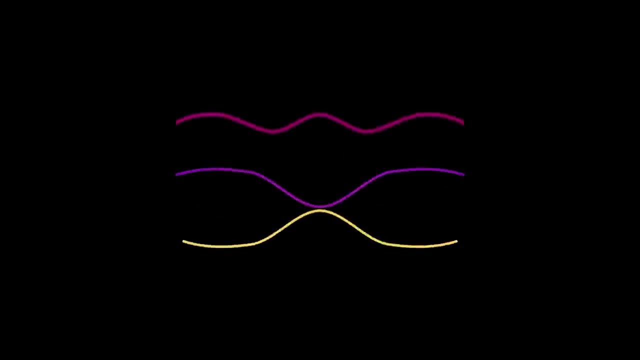 probabilities. A key difference is well, probability is always a number from zero to one. Amplitudes are complex numbers, And what this means is that they obey different rules. If I want to know the total amplitude for something to happen, I have to add up the amplitudes for all the different ways that it could have happened. 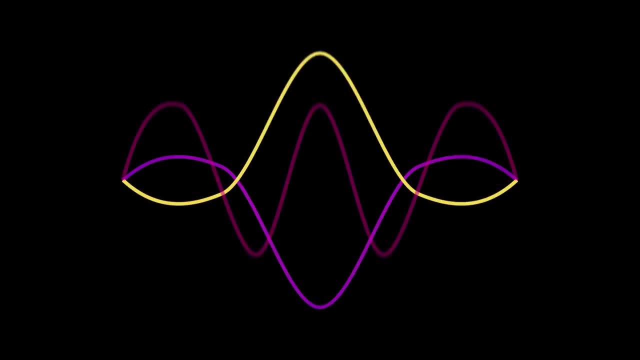 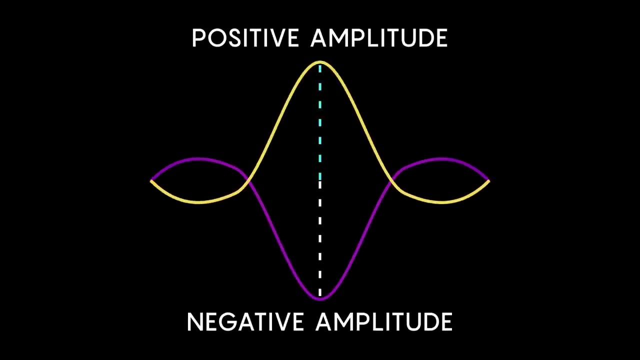 But when I add up amplitudes, I see something new, which is that a particle might reach a certain place one way with a positive amplitude and another way with a negative amplitude, And if that happens, then those two amplitudes can cancel each other out, so that the total amplitude would 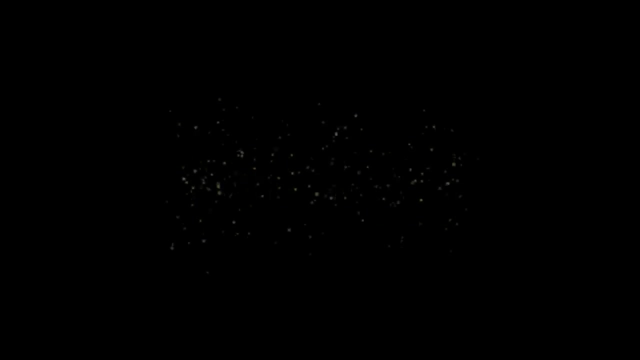 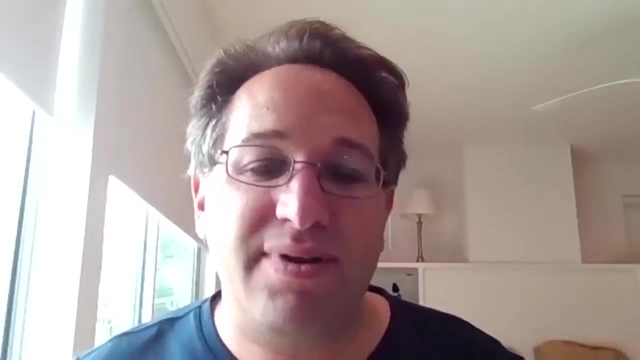 be zero And that would mean that that thing would never happen at all. This is sort of the central thing that quantum mechanics says about the world. right, That the way that you describe a physical system is by a list of amplitudes And the way that a physical system changes over time is by a linear transformation. 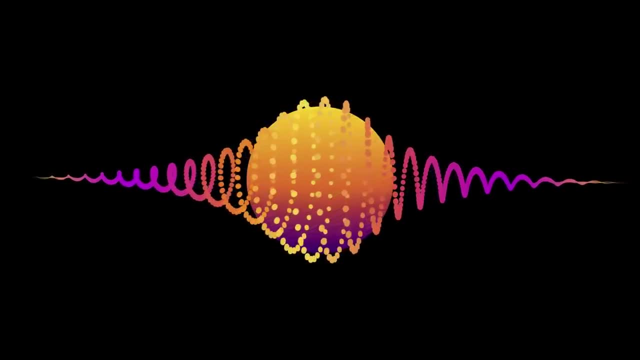 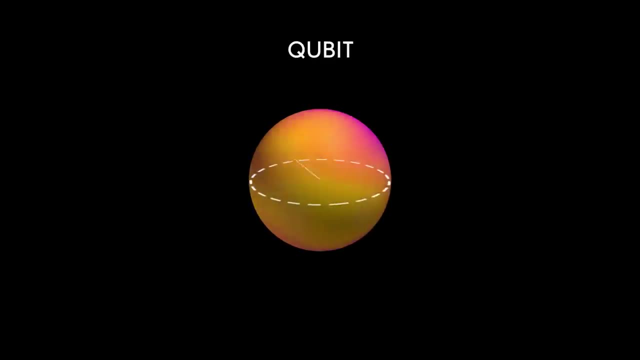 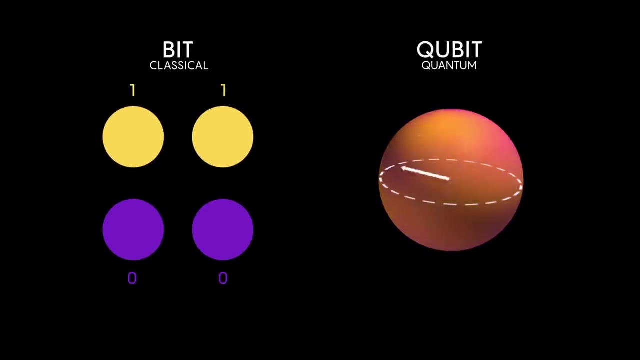 of these amplitudes. But how can quantum computers use amplitudes to store and manipulate information quantumly? This is a qubit. It's the basic computational unit in quantum computing. Qubits are like bits in a computer, but with a crucial difference. A bit is binary. It stores information in strings of. 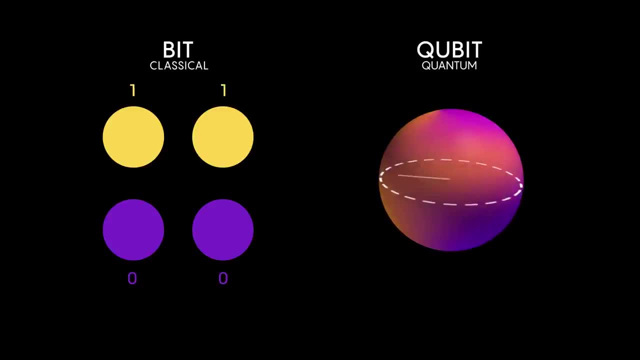 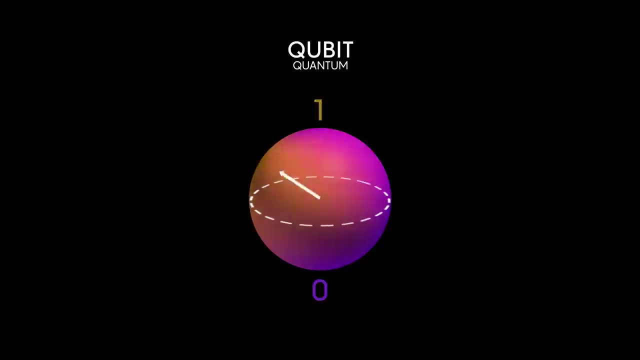 binary digits that can only be zero or one, But qubits are made of subatomic particles, so they operate according to subatomic logic. Qubits can be zero, one, or what we call a linear combination of zero and one. This fluid combination of amplitudes is at the core of quantum computing. 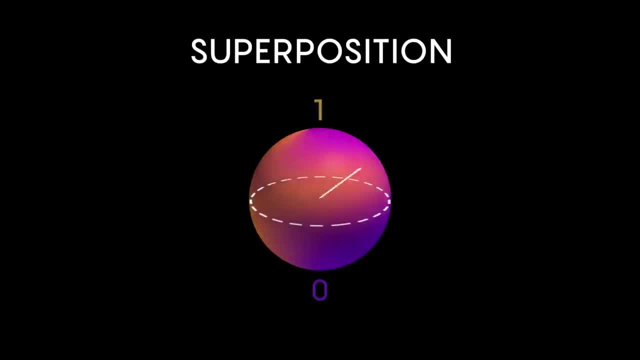 Before you measure a qubit, it exists in a state of superposition. You can think about it as a quantum version of a probability distribution where each qubit has some amplitude for being zero and some amplitude for being one. Superposition is the reason why it takes a vast number of classical bits to describe the quantum. 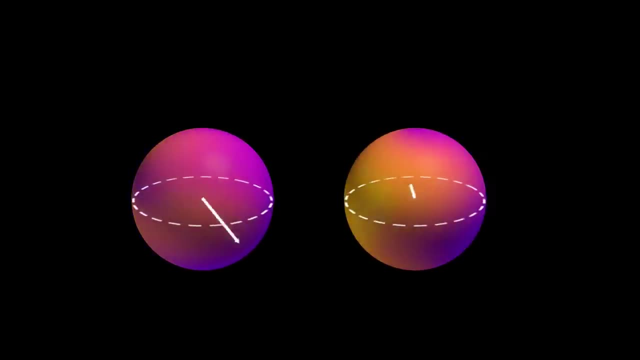 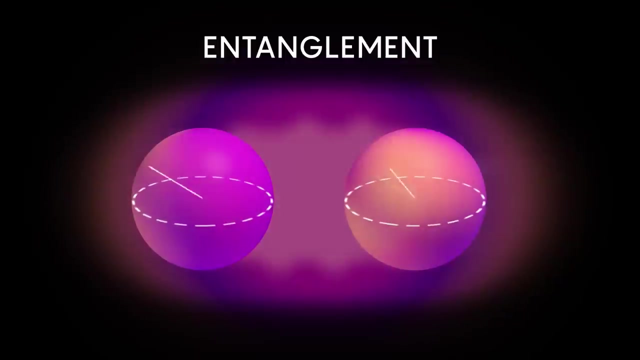 state of even a tiny number of particles. When two or more qubits are in this closed state of superposition, they relate to one another through the phenomenon of entanglement. This means that their final outcomes, when we measure them, are not the same as the final outcomes of the quantum. 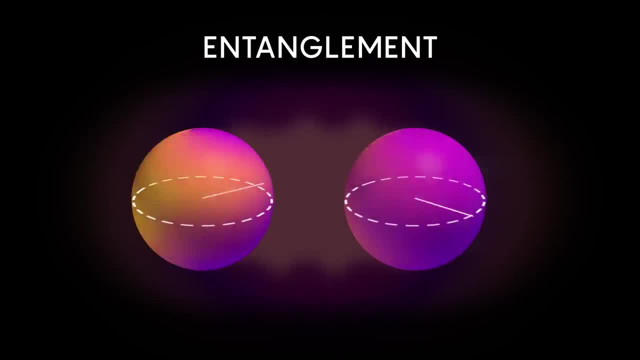 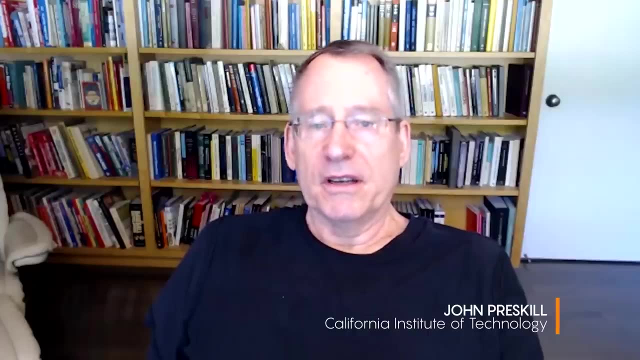 system. They are mathematically related. The key concept for understanding how quantum computing can be powerful compared to classical computing is what we call quantum entanglement, And that is the word we use for the characteristic correlations among parts of a quantum system. 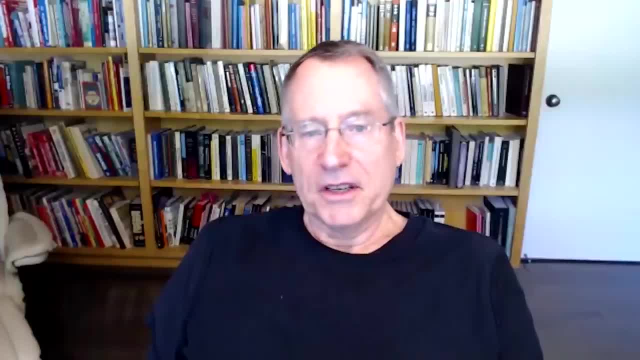 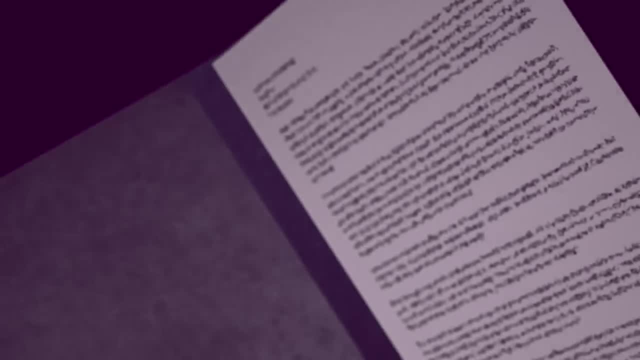 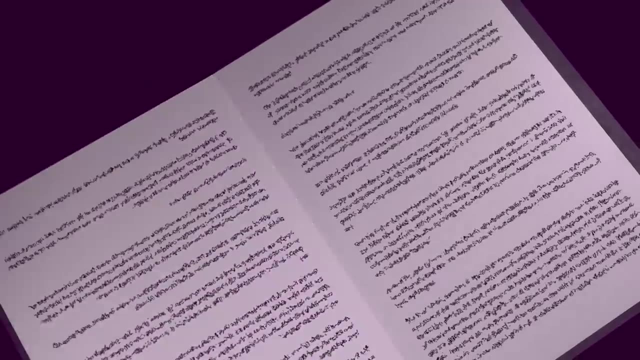 which are different from the correlations that we normally encounter in the classical world. in ordinary experience, You could think of it as is like a book. When you look at the pages, one at a time, you don't see any information, You just see random gibberish. 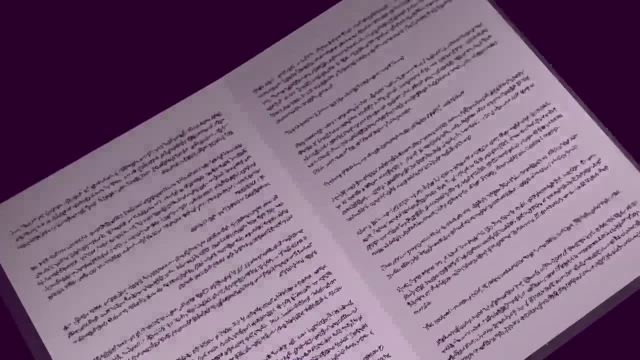 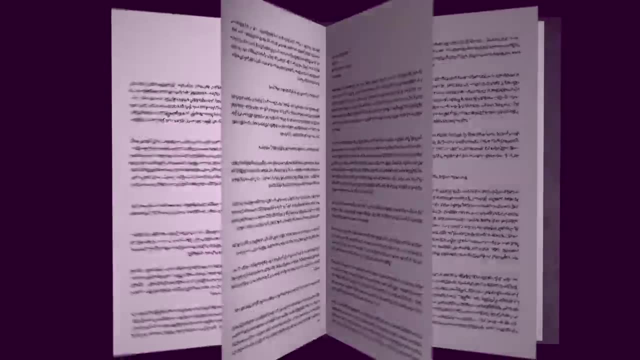 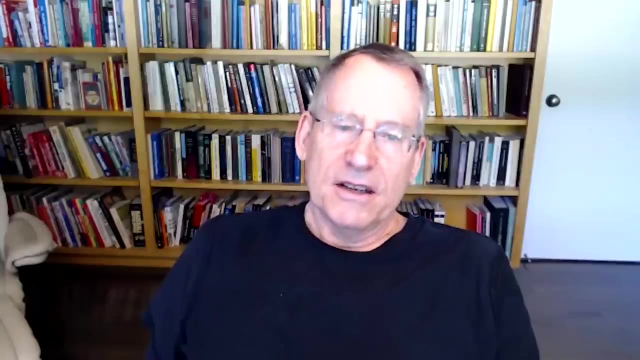 It's because the information isn't encoded in the individual pages but in the correlations among them, And to read the book you have to collectively observe many pages at once. It turns out- and this is part of what's so interesting- that if you want to describe very highly entangled states, 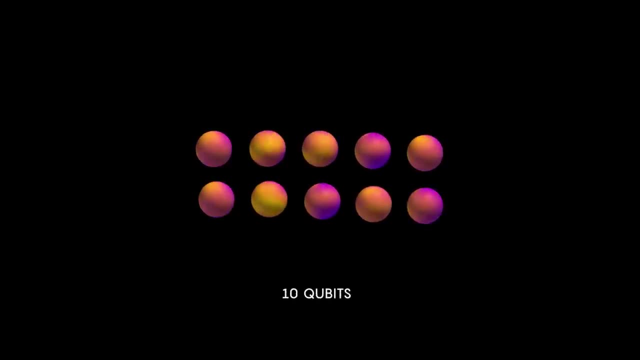 using ordinary bits. it's extremely expensive. Imagine that you had a primitive 10-qubit computer. It could store two to the 10th power values in parallel. To describe this entangled configuration with a classical computer you'd need two kilobytes or 16,000 bits. 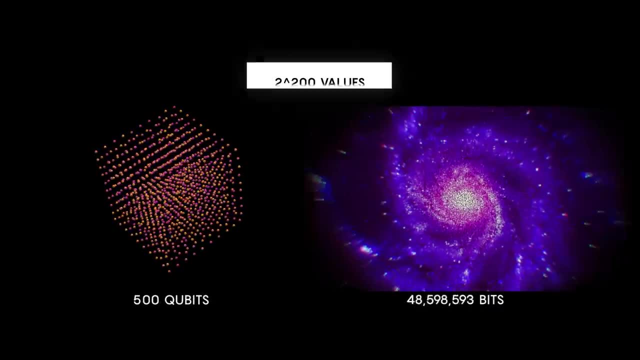 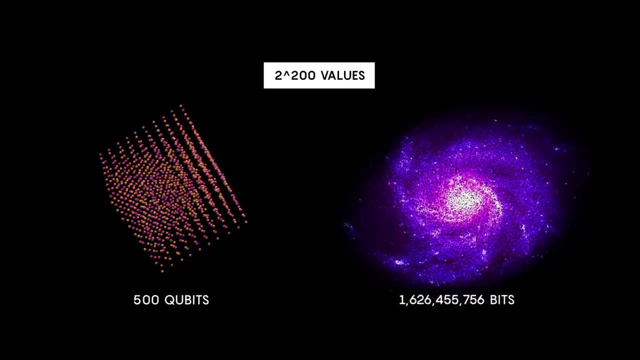 Expand to a system with 500 entangled qubits and you now require more classical bits than there are atoms in the known universe. This is exactly what Feynman meant when he said that classical computers weren't scalable for simulating quantum mechanics. For a quantum computer to be of any use, you need to measure information from the qubits to get an output. The problem is: when a quantum system is measured, it collapses into a classical state If anything carries away information about whether that qubit is zero or one. 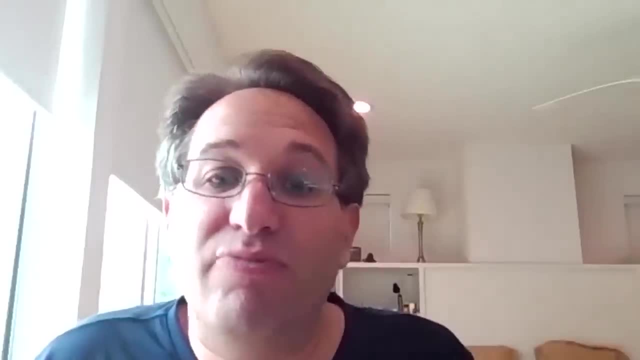 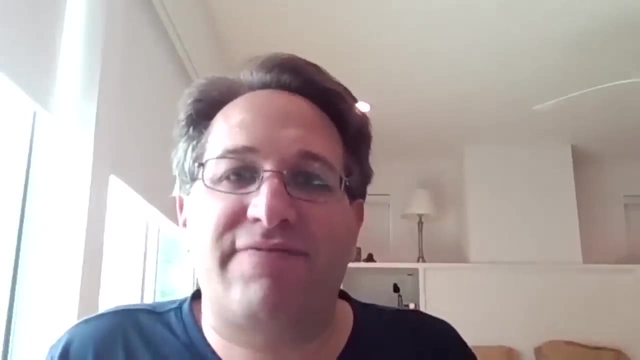 for example, if that information gets recorded in some radiation that's escaping from the quantum computer, then the effect on the qubit will be exactly as if someone had measured it To extract an answer from the quantum system. that isn't just a random outcome of probability. 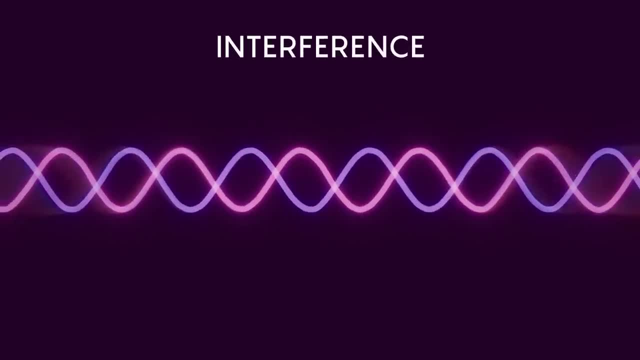 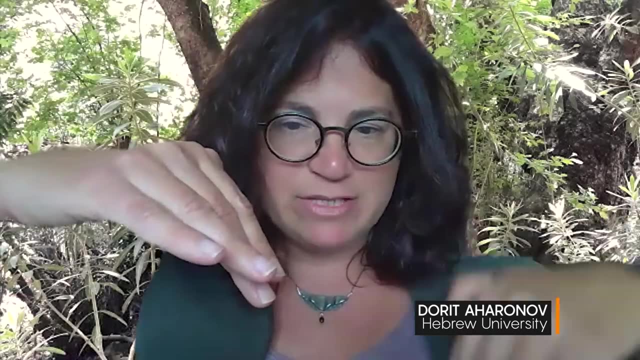 like the flip of a coin. we have to use interference. You can see interference when waves in a pool hit each other and one wave is above the surface and the other wave is below the surface and they hit each other and they cancel each other. 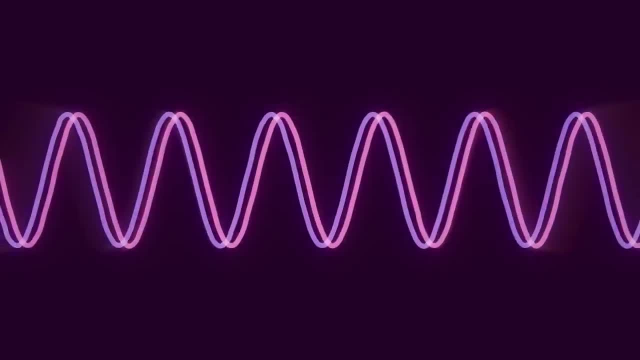 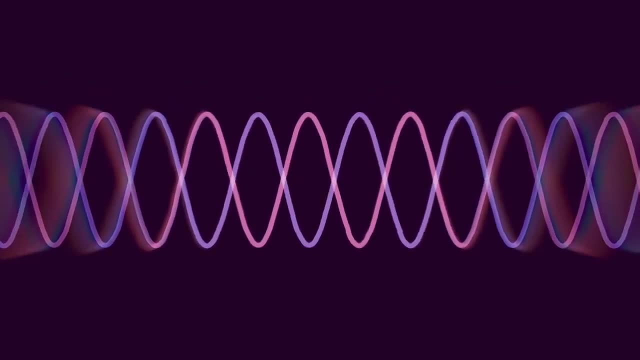 Interference is just what amplitudes do when you add them up. If something can happen one way with an amplitude of a half and another way with an amplitude of minus a half, then the total amplitude for it to happen would be zero. 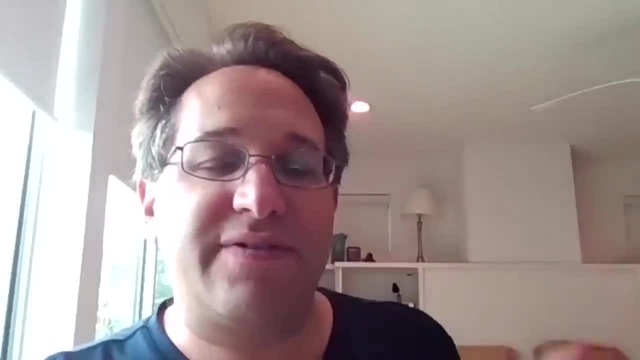 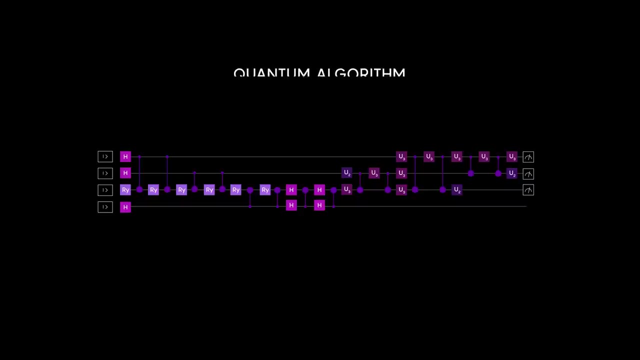 This is what you do in the famous double-slit experiment. You close one of the paths and then you see that now the thing that previously never happened now can happen. This is a quantum algorithm. Scientists can harness interference by creating a deterministic sequence of qubit gates. 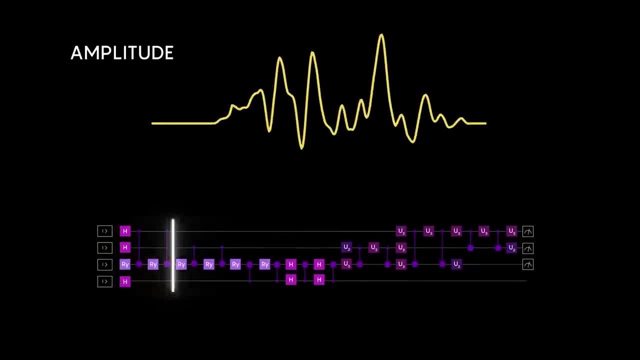 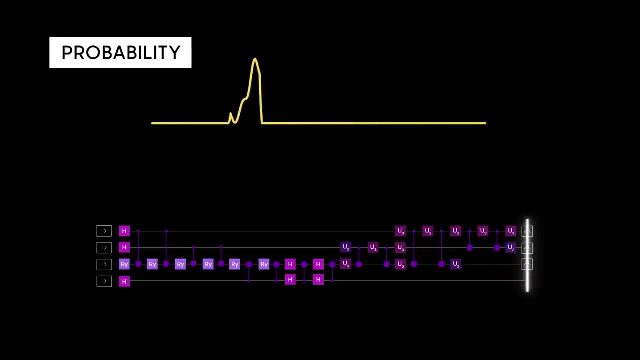 These qubit gates cause the amplitudes to add up constructively. This means that they're mathematically guaranteed to boost the probability of seeing one of the right answers. You might ask: how could you possibly concentrate all this amplitude on the right answer? 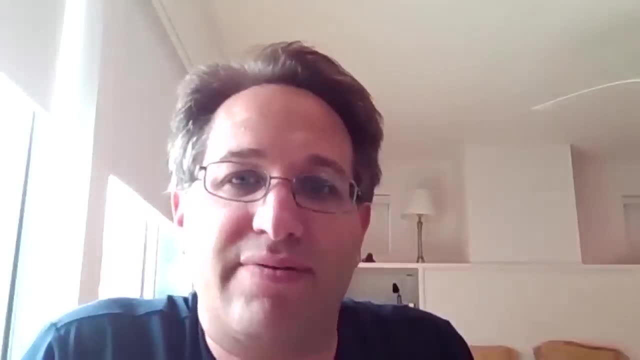 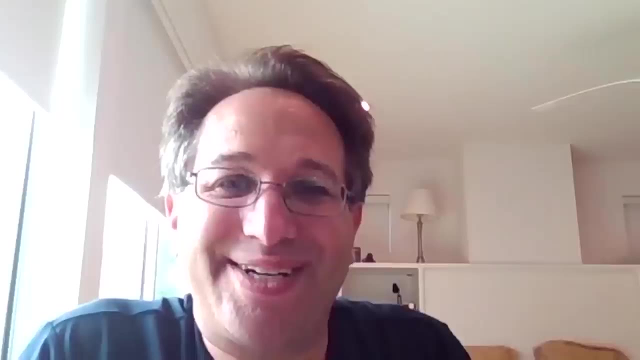 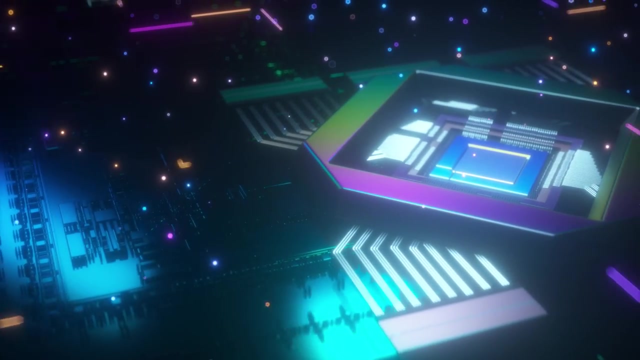 when you yourself don't know in advance which answer is the right one. This is exactly why designing quantum algorithms is so difficult and why we have a whole field that's been studying it for decades- Since 1994, there have been a few major breakthroughs. 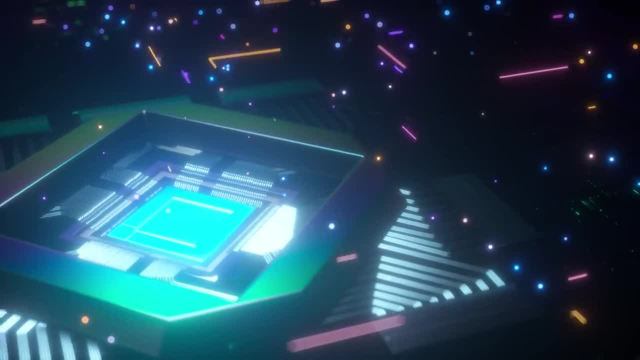 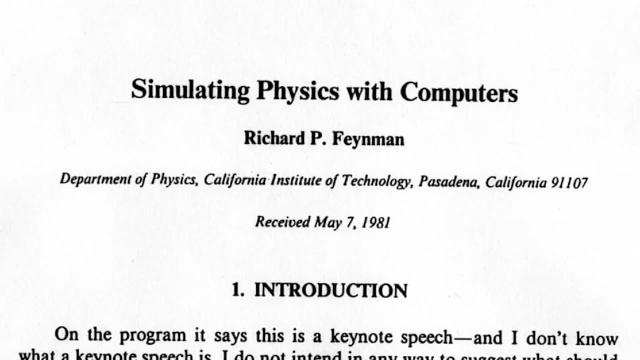 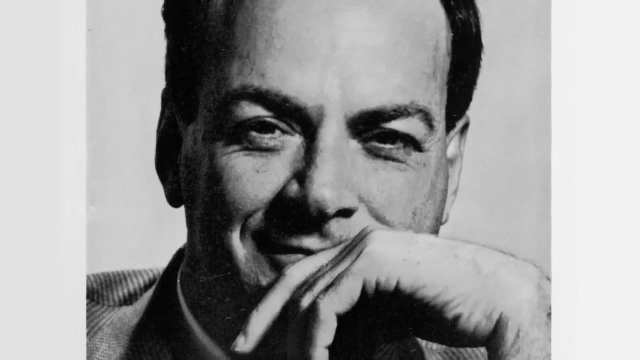 in quantum algorithms with theoretical applications in fields such as cybersecurity and search optimization, But according to most experts in the field, quantum computers are most likely to be useful for what they were born to do when a curious physicist wondered about the deep structure of our world. 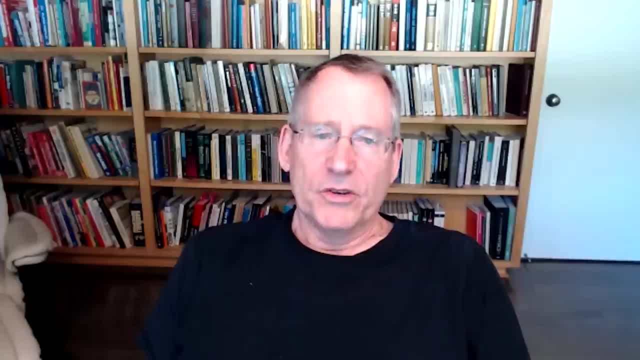 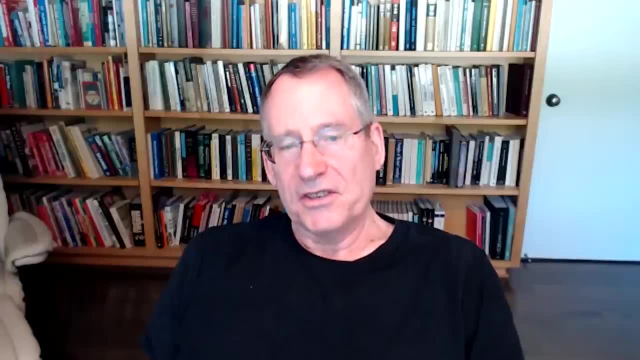 I find quantum computing exciting as a way to explore physics Now. whether that's going to make anybody any money, whether there will be practical applications in the near term, that's still very much an open question. But at least for physicists it's an exciting time. 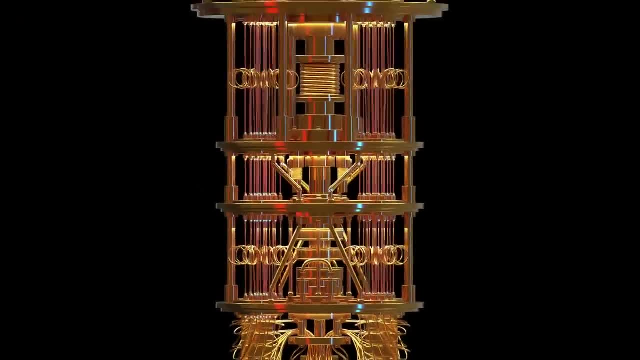 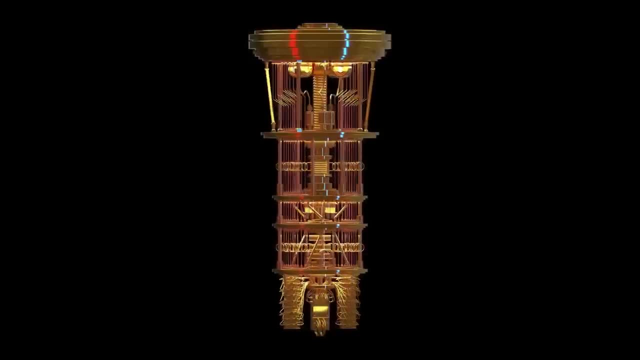 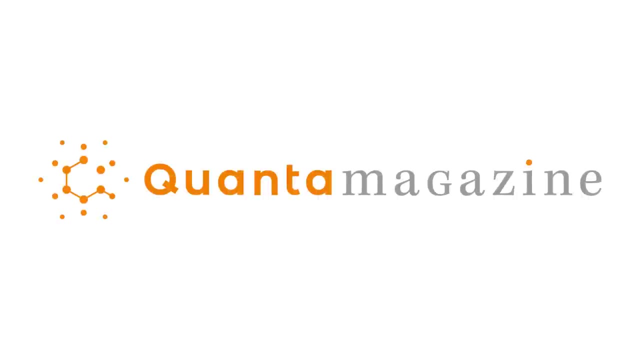 The truth is, the most important application, I believe, of quantum computers is something that we don't know yet. I'm sure that once we have a quantum computer to play with, we will find amazing applications that we can't yet foresee. NASA Jet Propulsion Laboratory, California Institute of Technology.